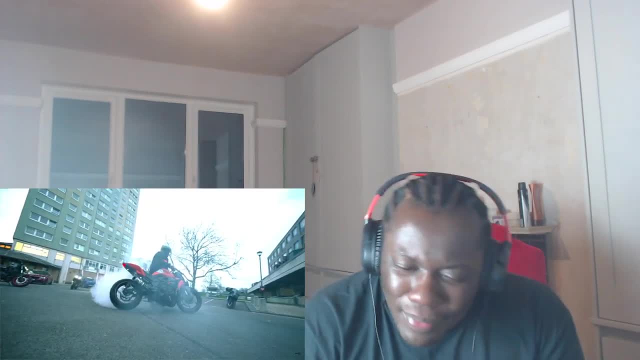 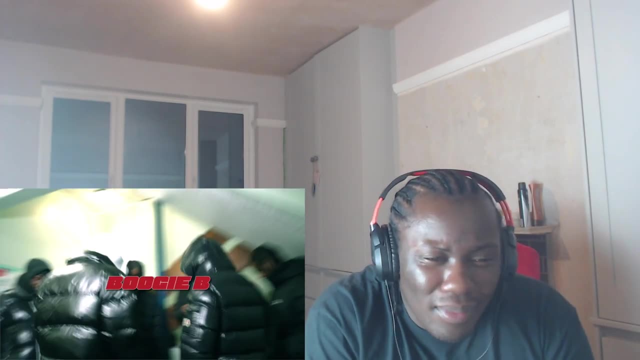 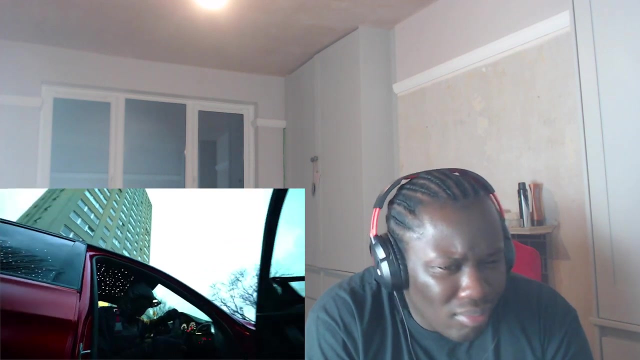 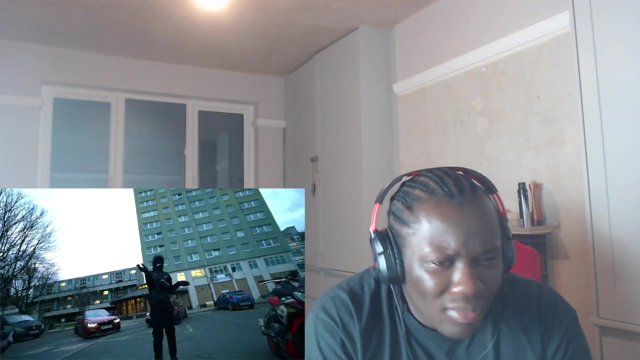 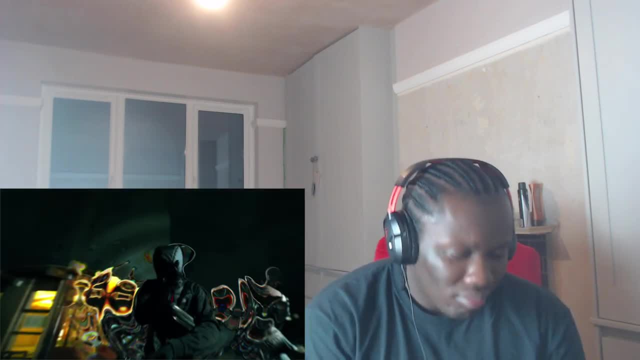 Where did that come from? Where are you dude People y'all? Oh, okay, Hey, I forgot to tell you You should leave. I was about to move. You got something in there. Get it, I got it. 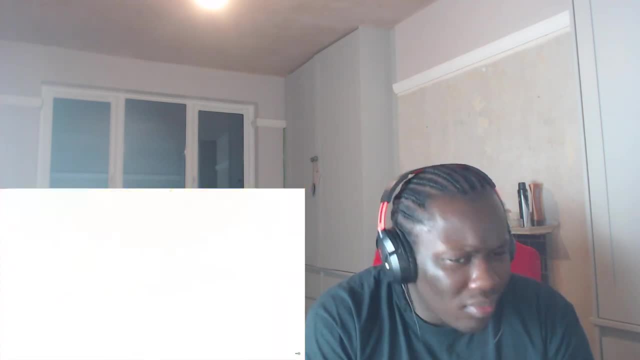 I got it. I'll take it. I'll take it. Okay, So now, what will we do? What's the plan now? How about we do this? We're gonna take this. So usually when we do this, we're gonna go for the club, so we're gonna have testing. 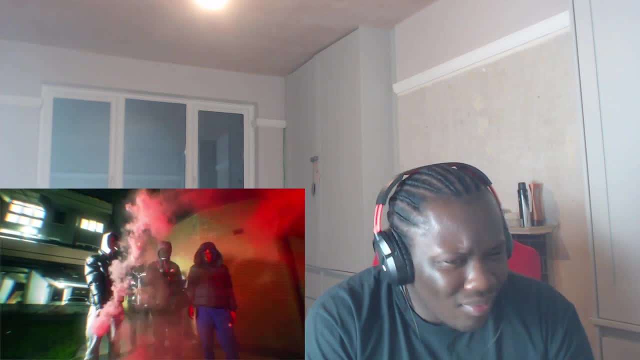 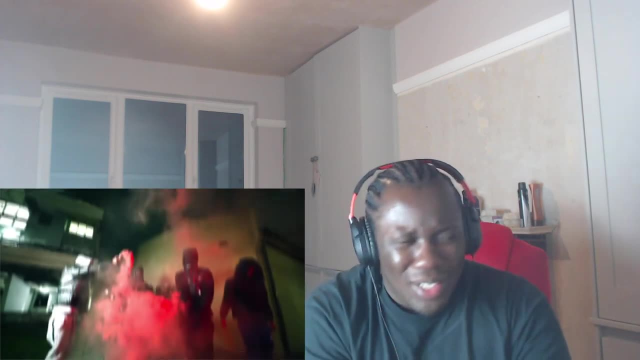 We're gonna do this, Yeah, But people just need to put it into: If you don't bring the fingers, kick it down, Your best duck will be cut round here. Don't run out of luck round here, Nothing. run out of luck round here. 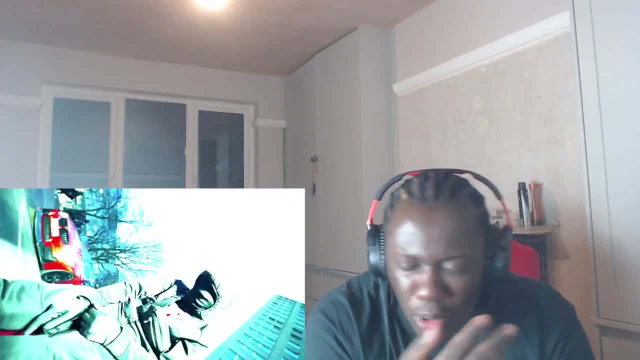 They had K's and they don't have K's. This is a serious algebra problem, But K can never equal an O. But when the O's had K's we finished the equation. That's, your bread drew B's make-all And six feet closer to the equator. 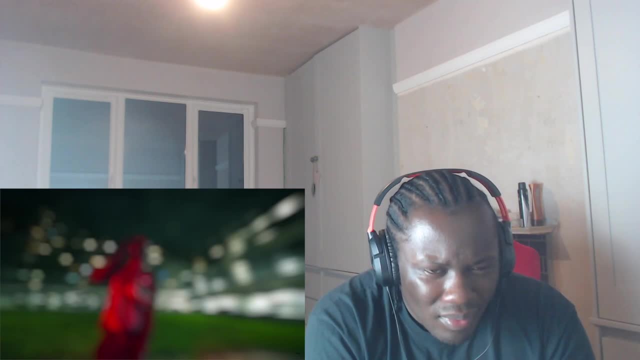 Like ha-ha, just know you're late Or not. literally when I bought this spiff And if I had a genie's butt I'd fling it to the ops And tell them: rub that shit And bring back their friends So we can pack them again. 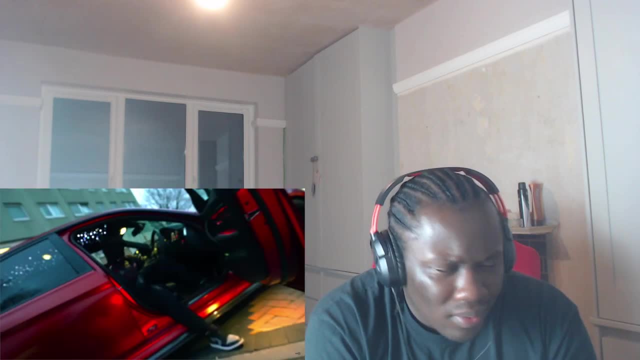 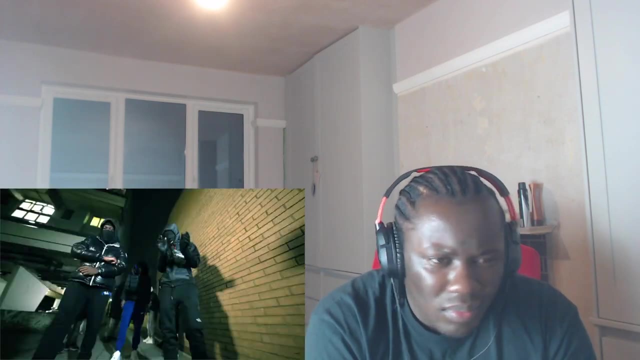 Slapped it. then I just slapped it again. I take the shovel and dig up your friends. Swing my angler arms at an angle, But I angle in a cute obtuse. I leave my flat line 180 degrees. Use that spinner, whip 180 degrees, Pop those, turn it up 25 degrees. 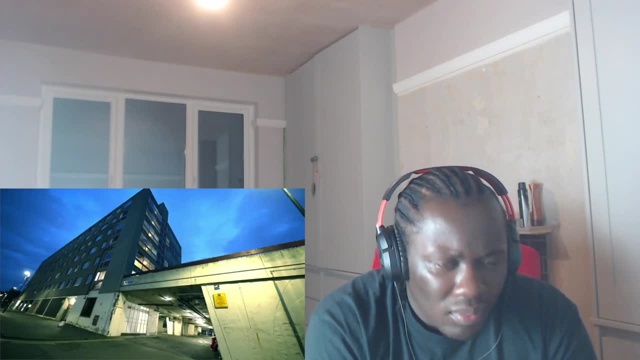 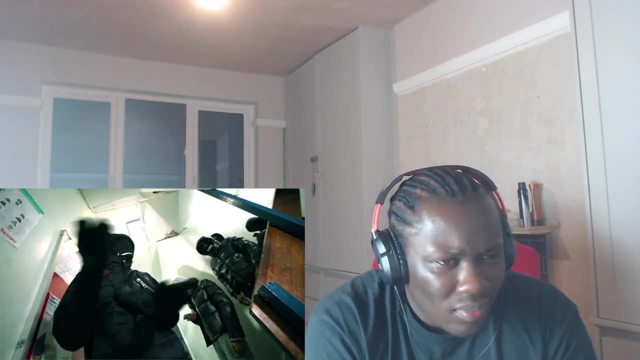 Had to cover my face like Like a nigga that'll sneeze. Had to risk being a man in the ground. Had to, Then it wouldn't be turning his grave And if reincarnation's real, They should come back as female dogs So they can be the black of the bitches they was. 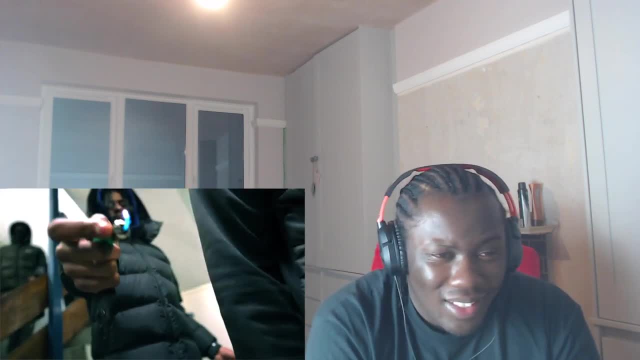 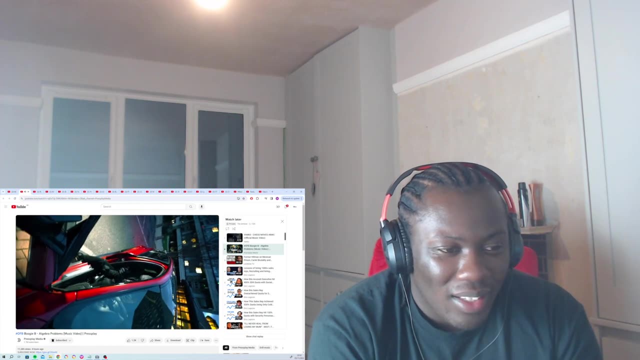 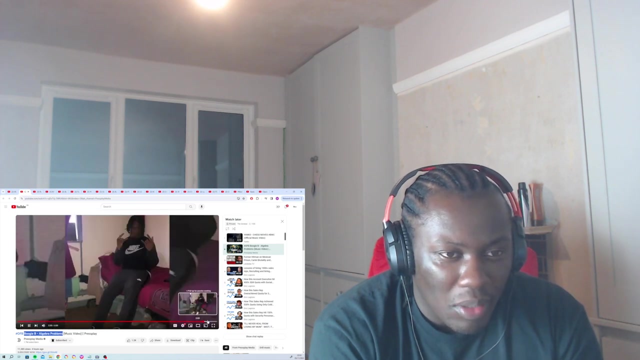 Listen to that, God, I owe it. You went crazy on this, though You went crazy on this. They that they, ah, nah, I can't lie that bar, That's one of the coldest bars a man has heard in a minute bro. 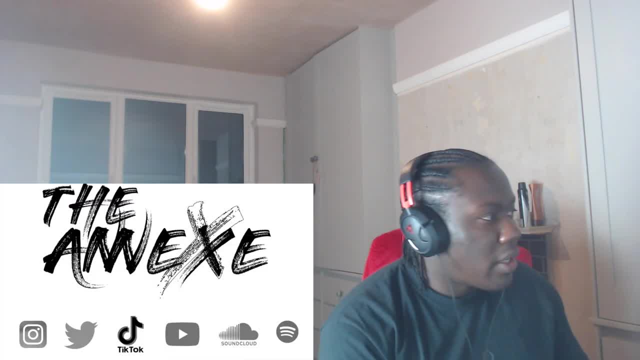 Free, free boogiebee though. But yeah, man, I can't lie that They add K's, but they don't have K's, Bro. that bar is sensational. That bar is sensational, bro. Yeah, man, they add K's to it. 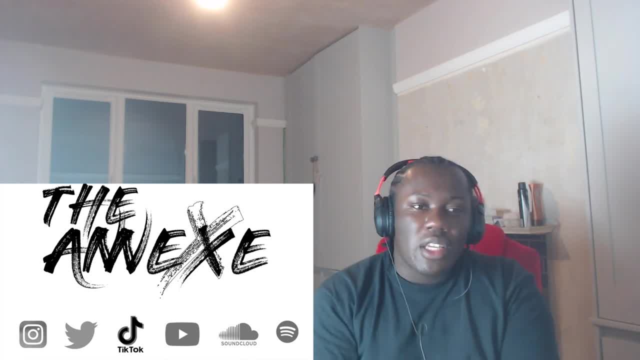 Nah, cold, cold, Finish. yeah, most man know that boogiebee's cold bro like Finish. yeah, most man know that boogiebee's cold bro like From that, um, from that verse He had bro, if I buck it up, 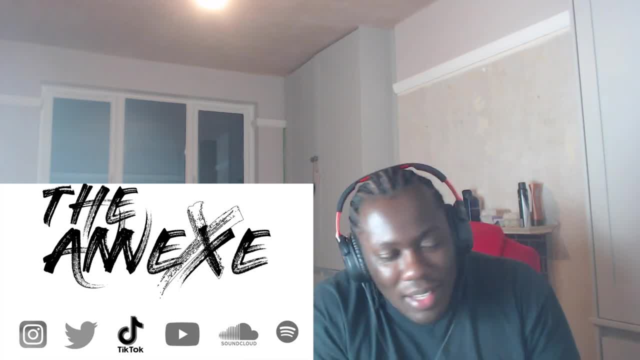 And I push it in then, bro, no homo, It's like, bro, like Everyone knows that boogiebee's cold and he's had a few other Mid-features as well on like exclusives On one or two tracks. so 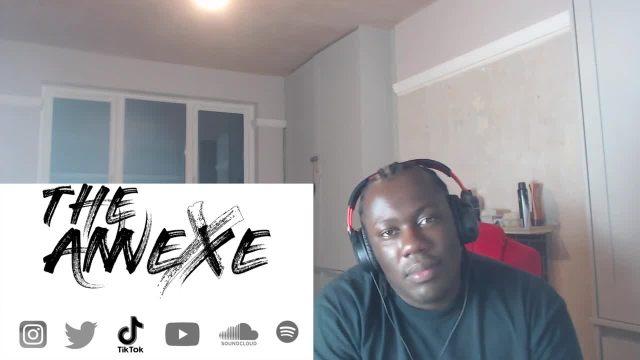 Brothers know you could rap, but obviously Things happen and yeah, man, It's a bit peak, but I can't lie. It's a so-called drop man. maybe you can do the Man's Manointing where you just drop the bare music from gel. 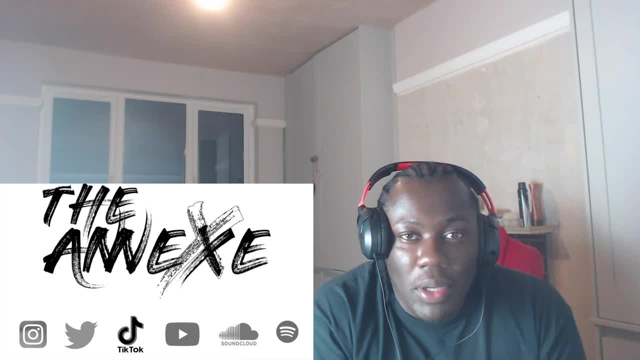 And then Just releasing the bare gel from this one, Like Mazda L20 will be releasing music from gel For years, bro, for years. So it's an angle, bro. it's an angle. I don't know how them man do it, but 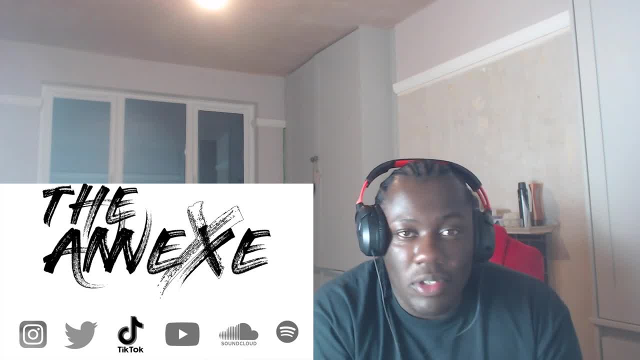 Bro, just give their engineers And then their mixer masters a raise innit. But yeah, you, man, let me know Your thoughts on this one. I thought it was a cold tune And yeah, man, I'ma stay posted. I'll catch you on the next one. 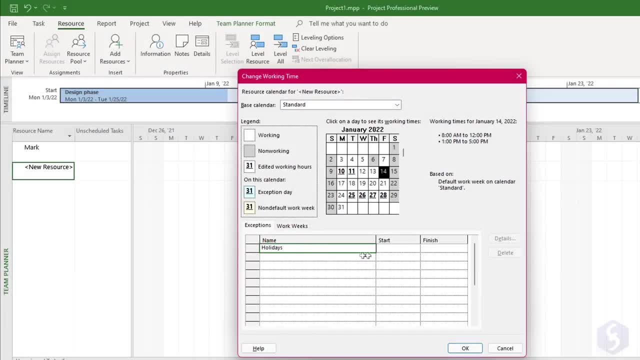 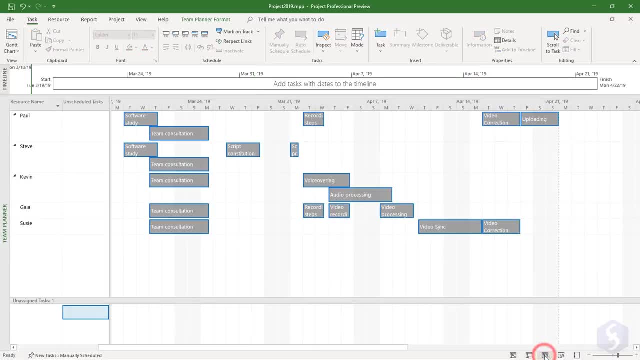 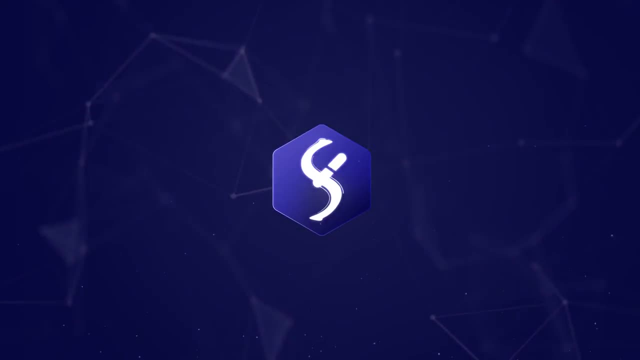 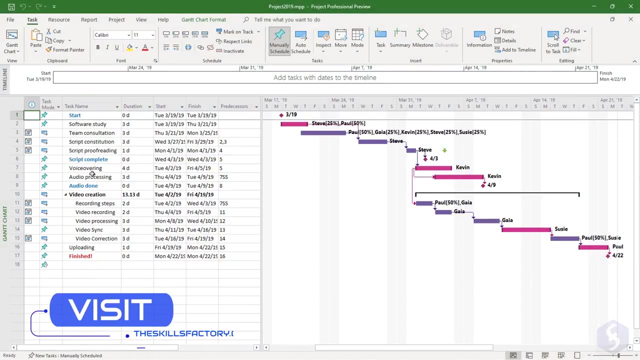 Dear all, welcome to this new tutorial dedicated to Microsoft Project. In just 14 minutes, we are going to see everything you need to know to start using it. even if you see it for the first time, Microsoft Project is one of the best project management products available. 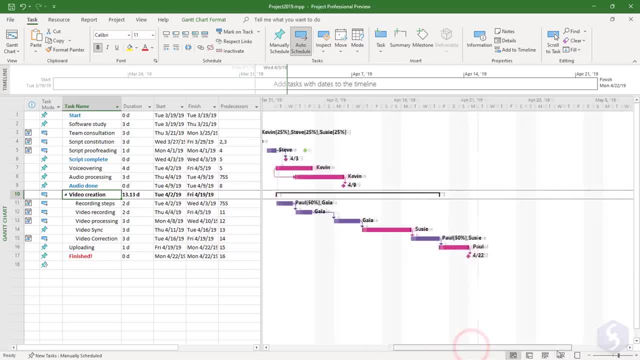 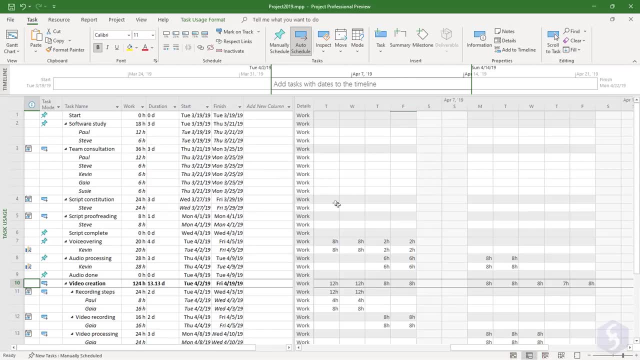 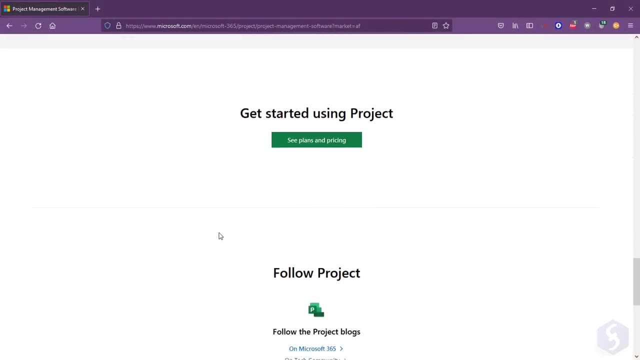 Once you define working times, holidays, people, resources and deadlines, Project helps you get the best solutions to respect the deadlines, reduce the expenses and reach milestones. Project runs on Windows 10 and 11 and is available as a cloud subscription plan or a perpetual license on its own. 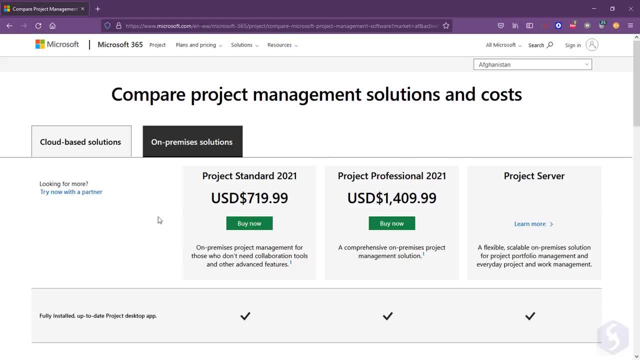 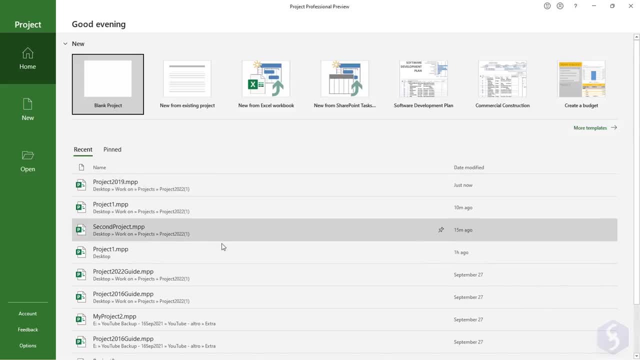 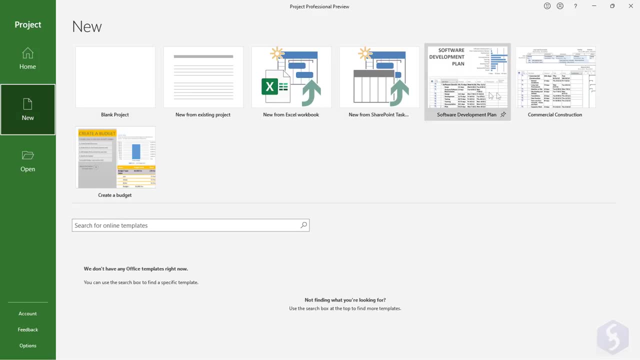 since it is not within any Office or Microsoft bundle. When opening Project, this shows several options for you to choose from. For example, you can choose from multiple options to start working. You can reopen any existing project in an MPP format or pick any ready template offered by Microsoft.